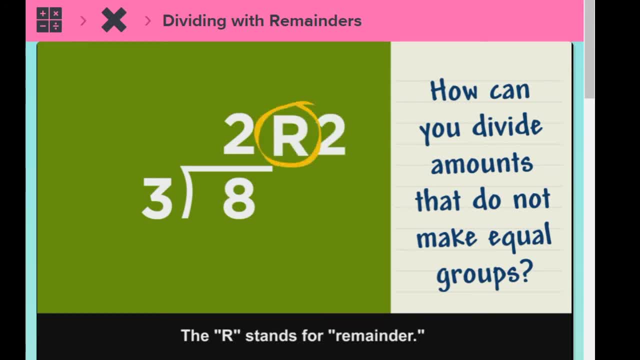 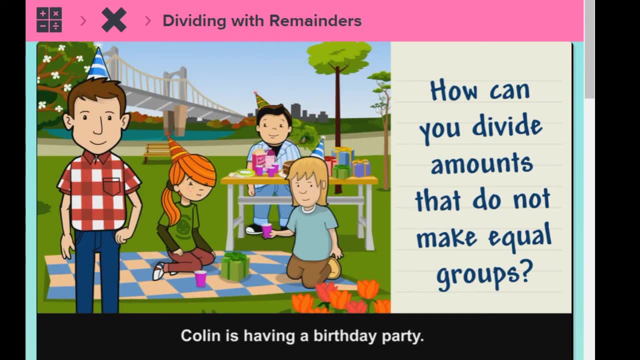 The R stands for remainder. The R stands for remainder. The R stands for remainder. Colin is having a birthday party. Colin is having a birthday party. There are seven party favors and there are four cards. There are seven party favors and four people. 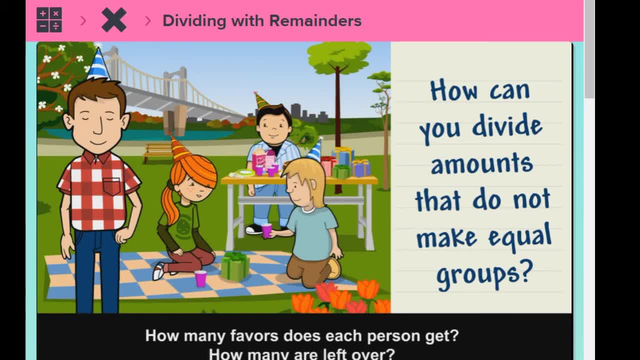 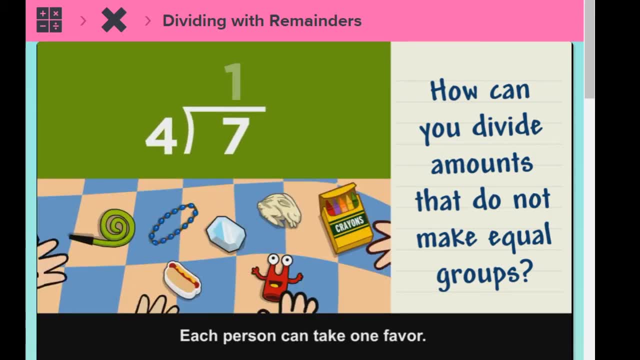 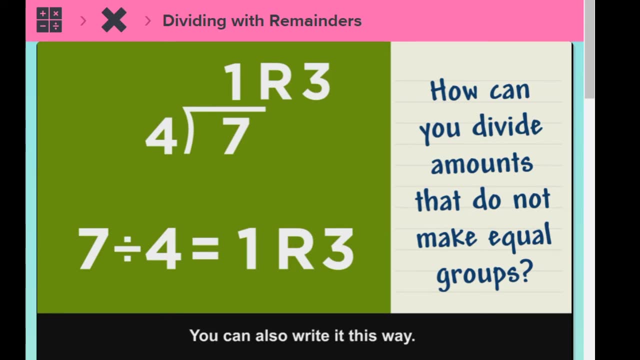 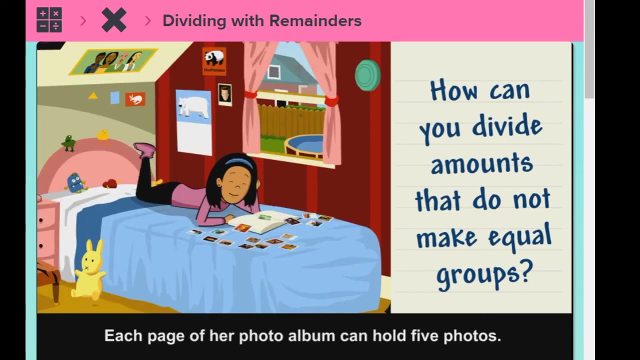 How many favors does each person get? How many are left over? To find out, divide seven by four. Each person can take one favor. There are three left over. You can also write it this way: Mia has sixteen photos. Each page of her photo album can hold five photos. 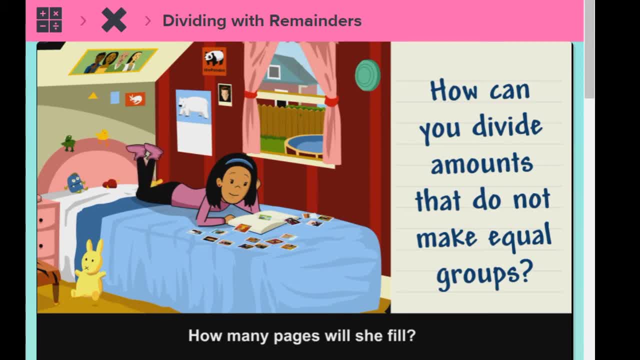 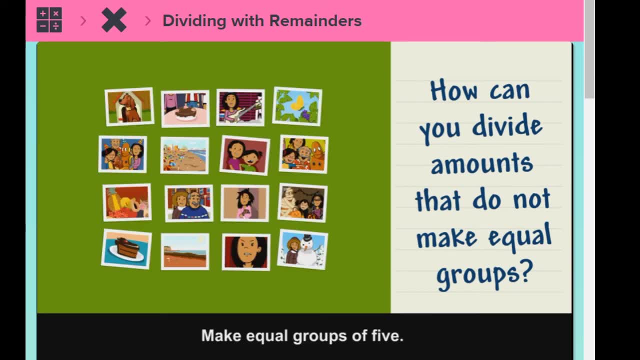 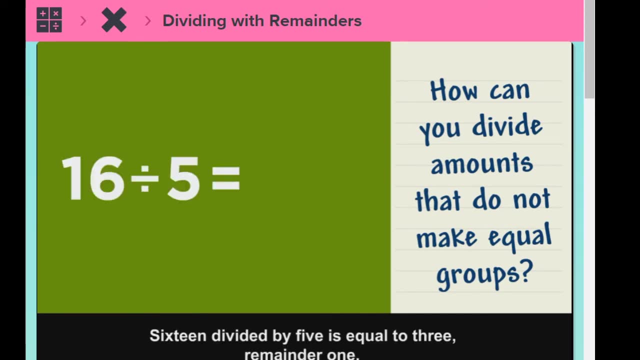 How many pages will she fill? How many photos will be left over? What is sixteen divided by five Make equal groups of five. There are three equal groups and one left over. Sixteen divided by five is equal to three remainder one. 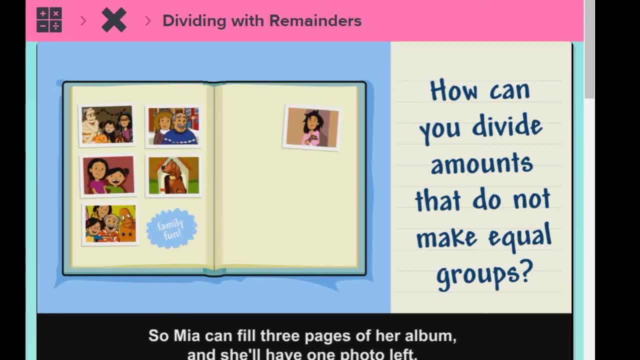 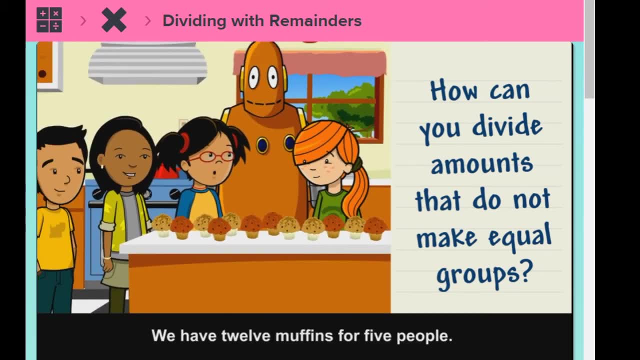 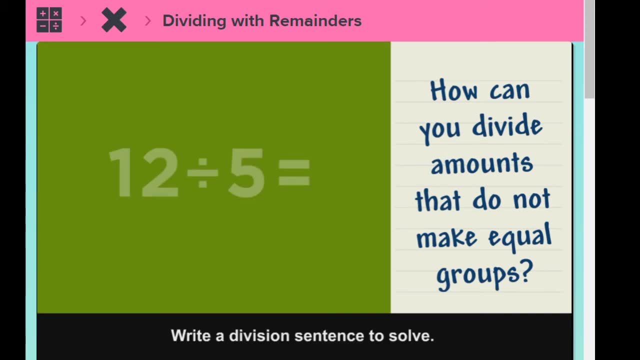 So Mia can fill three pages of her album and she'll have one photo left. We have twelve muffins for five people. How many muffins do we get each? How many are left over? Write a division sentence to solve. We can make five equal groups of two. 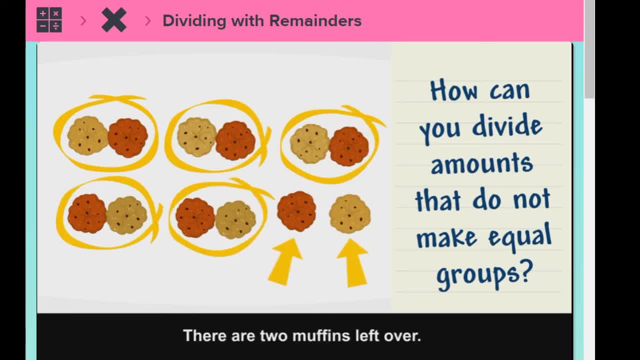 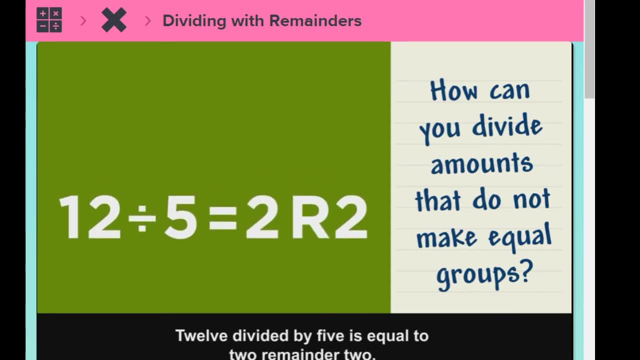 There are two muffins left over. Twelve divided by five is equal to two remainder two. The twelve stands for the total number. The five stands for the number of groups. The two tells you how many are in each group. The remainder tells you how many are left over. 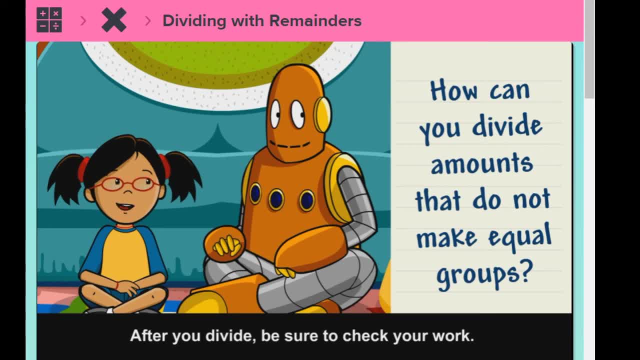 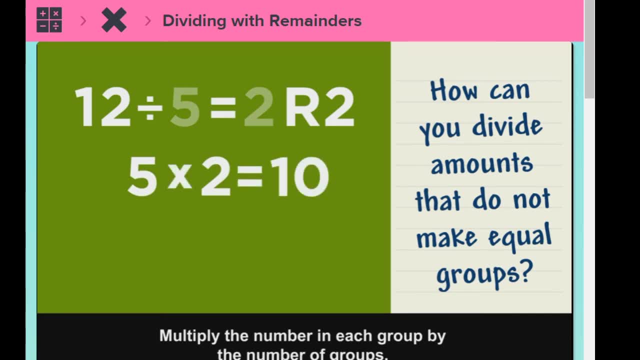 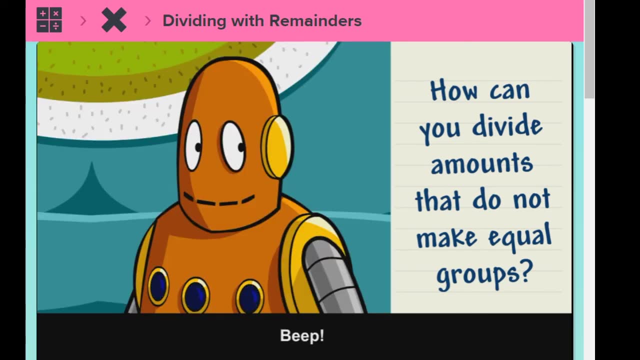 After you divide, be sure to check your work. Multiply the number in each group by the number of groups, Then add the remainder. The answer should be the total number. There are twenty six. There are twenty seven robots. Each shelf holds six robots.